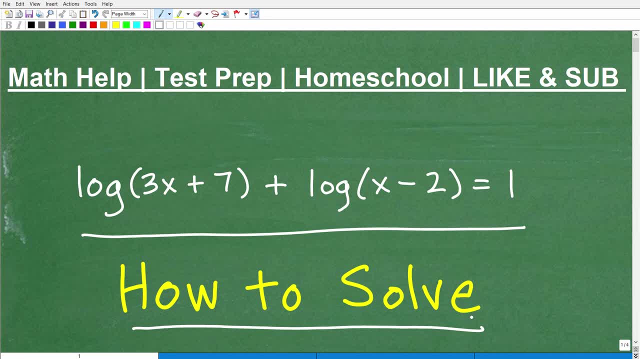 and you're struggling. well, you got to first start working harder, Okay, but the second thing you need to do, or need to be successful in mathematics, is great math instruction: Clear, understandable, comprehensive. That's where I can help you out. So if you're at the middle school, 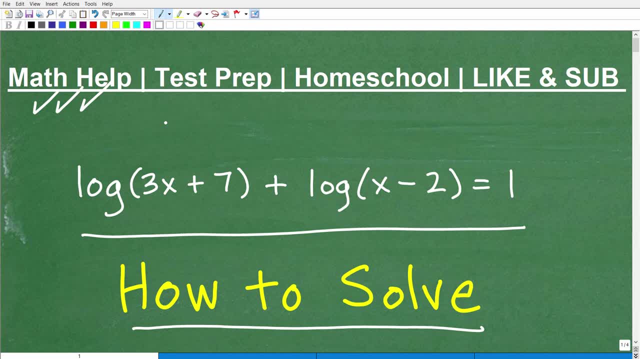 high school or college level. check out my math help program. I'm going to leave a link to it in the description of this video. It will help you out tremendously. Also, if you're preparing for any sort of test with a math section, something along the line the GED, SAT, ACT, GRE, GMAT. 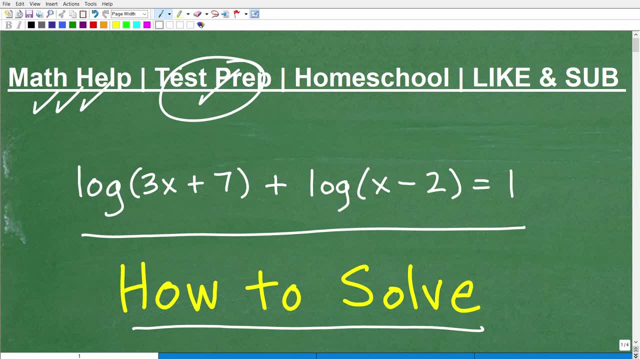 maybe the ASVAB or teacher certification exam. I have a ton of test prep courses that I can help you out. If you homeschool, I have excellent middle and high school math courses for homeschoolers And if this video helps you out, consider helping me out by liking and subscribing to my channel. 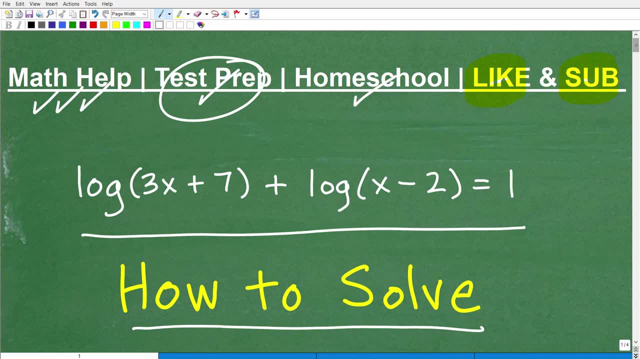 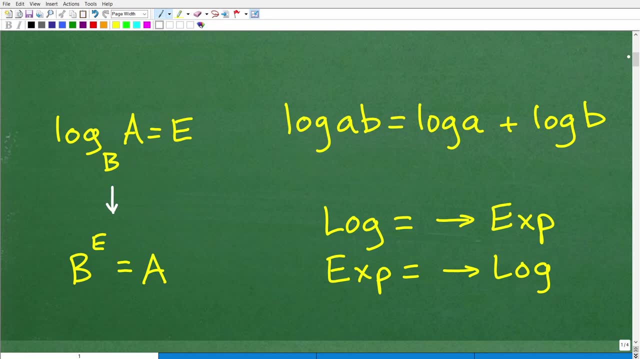 All right. so let's get into this problem And let's first of all just talk generally about to know for this particular problem. just you know basically how do we solve a logarithmic equation? So the first thing you need to understand. let's kind of start over here. 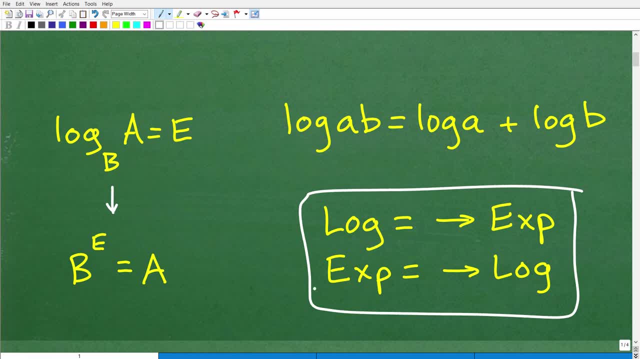 actually is that when you solve an exponential equation, something like this: 2x is equal to 7, this is an exponential equation because our variable is an exponent. okay, Well, an exponential equation. when you have an exponential equation, you're going to use logarithms to solve that. 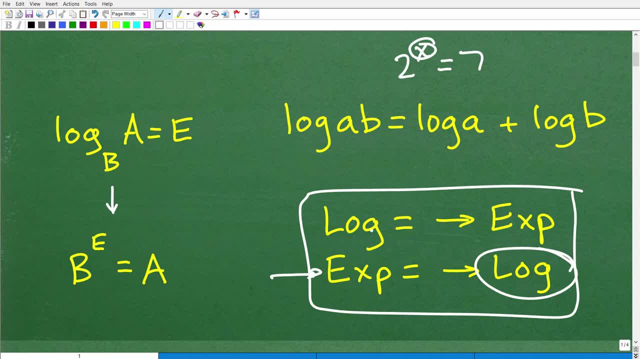 okay. Now, exponential functions and logarithmic functions are inverses of one another. So when you're dealing with a logarithmic equation, you're going to be using exponents and k powers, all right. So that's the first thing you need to be thinking about is like: oh, I'm dealing with a. 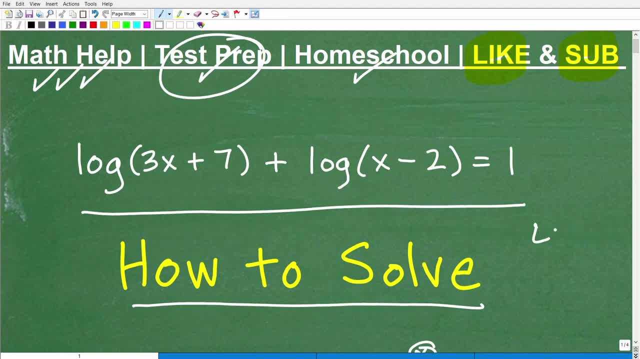 logarithmic equation. What am I going to be using? Am I going to be using my LOG button on my calculator? No, the answer is no. What you need to be thinking is: oh, I see LOG or LN, that's the. 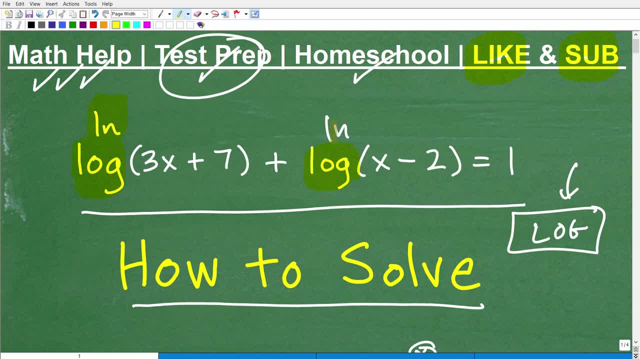 LOG. okay for those of you out there studying that, If you see any of these things, you're going to think to yourself: wait a minute, that guy on YouTube told me to be thinking exponents, exponential functions, and that's exactly what you want to be thinking. And then, when you see, 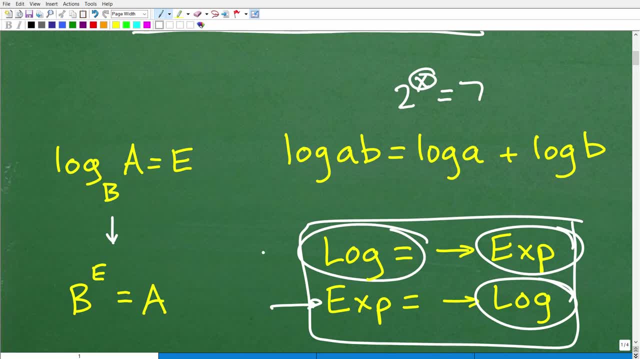 an exponential equation. you want to be thinking logarithms, So you know you got to be thinking the inverse, right? So that's the first main concept here. Now, the way we convert a logarithm or the way we rewrite it as a power, okay, or an. 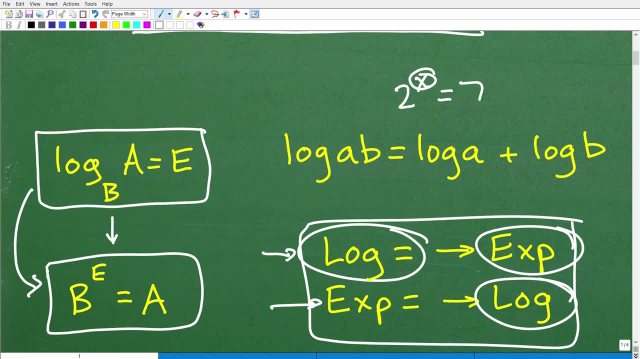 something that involves exponents is one of my favorite sayings in mathematics, and that's bacon and- and I'll run it out here- eggs, bacon and eggs. And you're like saying: all right. some of you are probably like: oh my goodness, why am I even listening to this guy on YouTube? He's talking. 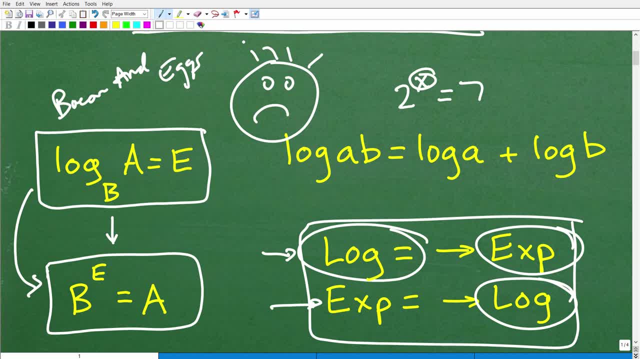 about bacon and eggs. He's probably hungry. He hasn't had his breakfast yet. Well, listen, I'm telling you something very, very important here that will help you out. So when you have a logarithmic written out log and you have some stuff here equal to some other stuff, Well, what this is, 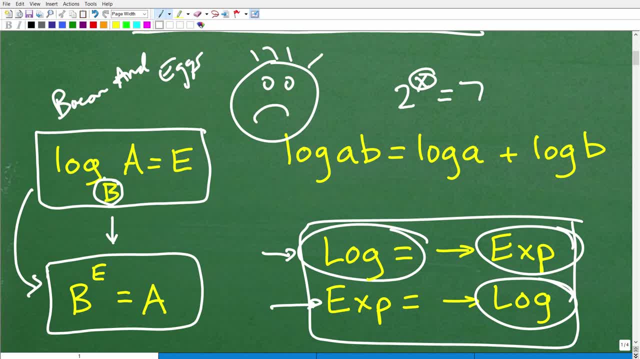 this little bead number down here, okay, this little number, this subscript, that's the base, This is the answer, And this little E, okay, is the exponent. So you kind of think of this as bacon and eggs B-A-E, which means that you can write, rewrite a logarithmic expression as an 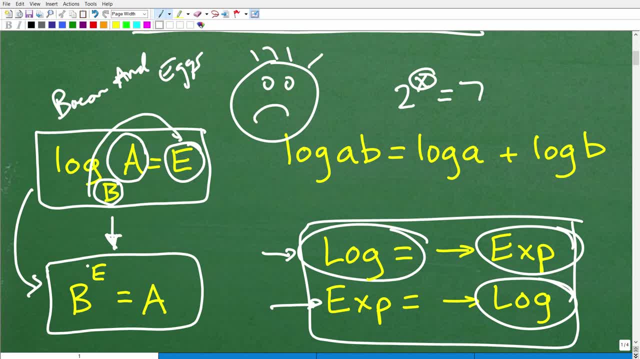 exponential or a power expression by going: okay, the base, right like two to the fifth power is equal to what 32, right? So two is the base, five is the exponent and the answer is 32.. So the base to the little exponent is equal to the answer. So 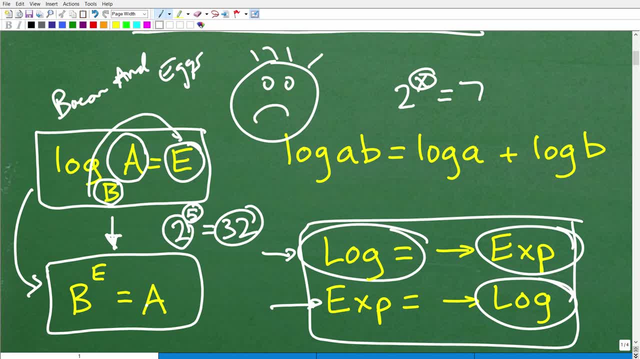 you just shuffle these things around and that's how you write a logarithm as a power. okay, Just remember bacon and eggs. whoops, bacon and eggs. Let's just go ahead and highlight this here for you. So, if you've never realized that, or you know, if you're always confused about that, 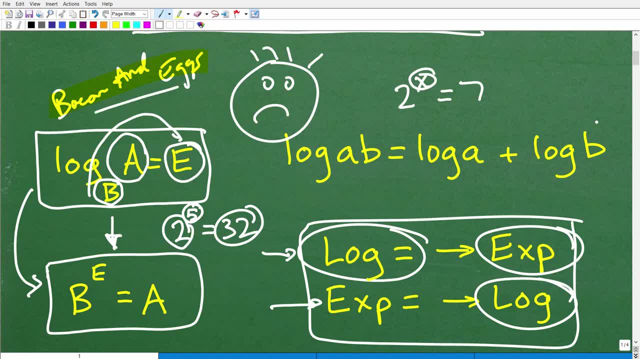 hopefully, this little mnemonic will help you out. Okay, now, the other thing we're going to need for this problem is we need to understand some of the properties of logarithms. There's other ones, but this is the one that we're going to be using right here, And it's- I believe it's- called the. 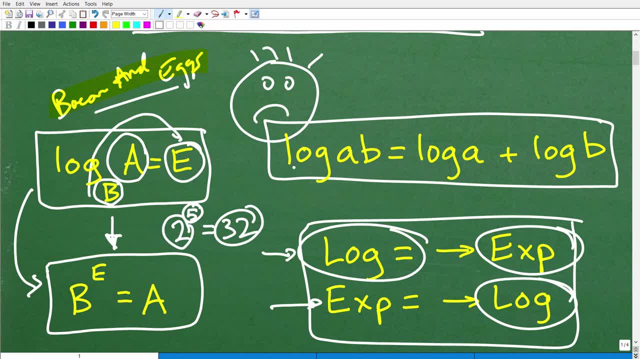 product property of logarithms. but basically works like this: When you have the logarithm of a product, like the log of A times B, you can separate these, these two factors here, by addition. okay, Now when we have a logarithmic expression, 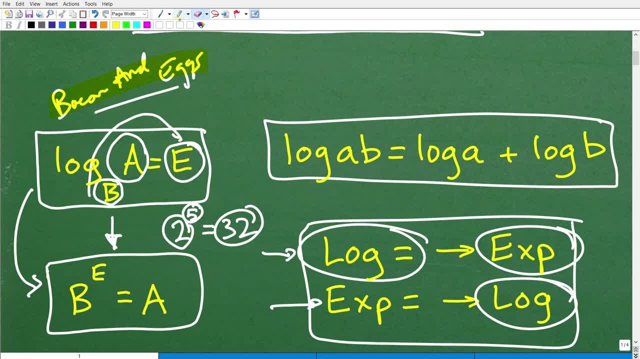 let me erase this guy right here. like this: log A times B, and we're going in this direction, you would be what we call expanding this, expanding this expression. So if I told you to expand log A times B, you could write it as log A plus log B. okay, That's called expansion. 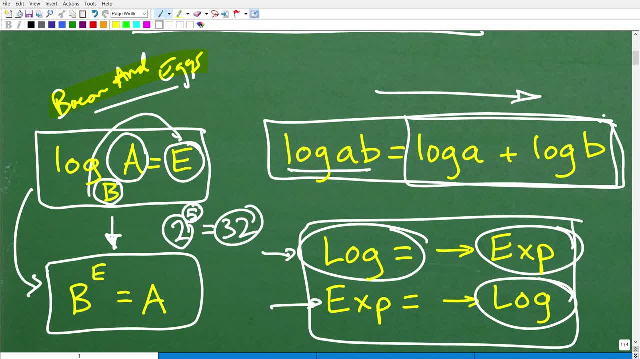 If I give you this- I said condense or rewrite this log A plus log B- you would go the other way and you would give me log AB. So you need to know how to expand and condense. Again, these are properties of logarithms, so you got to understand. 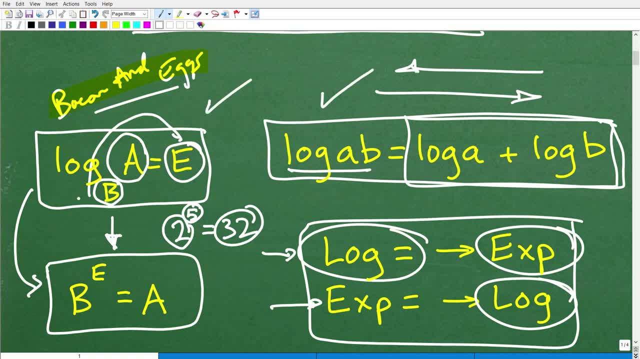 that You got to understand bacon and eggs, how we can write logarithms as powers, And you also have to see the big picture that when you're dealing with a logarithmic equation, we need to be thinking in terms of powers, exponential functions. okay, All right, so that's the big 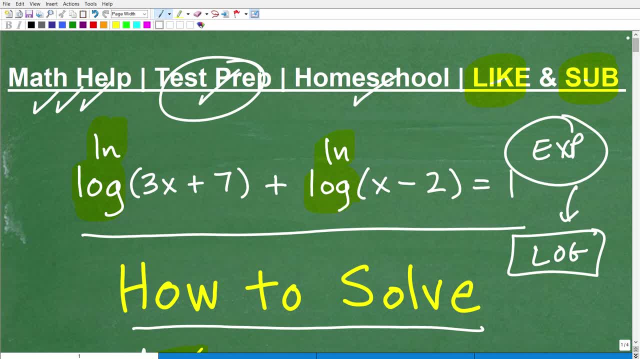 picture here And if you're like, okay, I understand. Well, if that's the case, that's fine. But if you're like, okay, I understand, Well, if that's the case, that's fine, Go ahead and tackle this problem Again. you're not going to need a calculator, just going to. 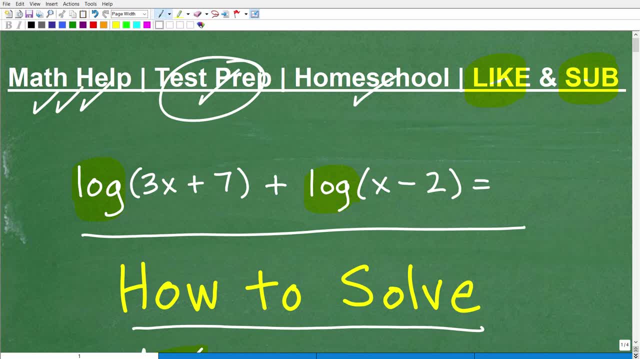 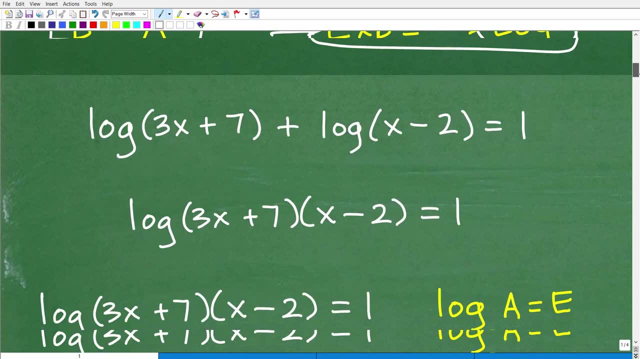 need the. well, you will need the calculator, the one between your ears, But again, not that difficult of a problem, Okay. so now let's go ahead and tackle the equation right now. Okay, so the first thing is- and by the way, this is a little bit more advanced and tip near more basic: 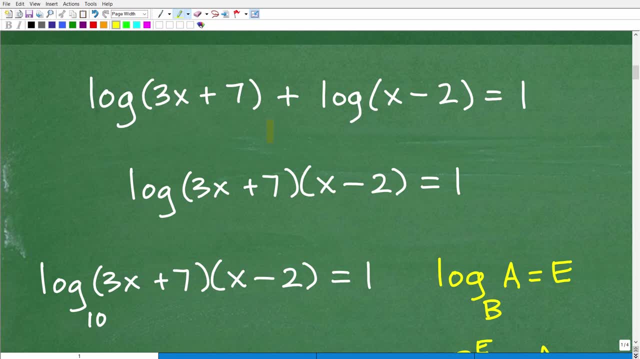 logarithmic equations. So if you're kind of like, I just need to learn this, but this one, this problem is too difficult for me. Let me give you a couple of suggestions. One: I have a ton of videos on my YouTube channel that I where I solve logarithmic. 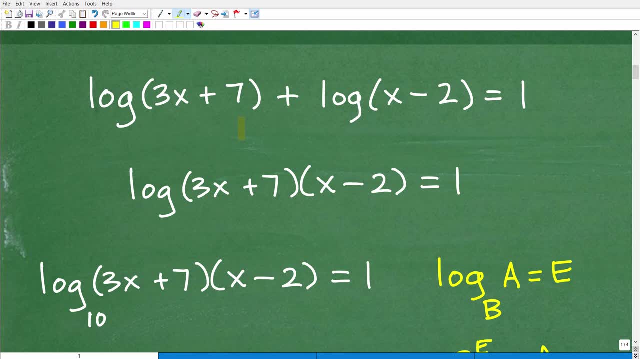 equations that can help you out. But two: you definitely want to check out one of my math courses and my math help program, algebra two, college algebra, pre-calculus. get into this super thoroughly. All right, so here we have log. okay, three X plus seven plus log of X minus two. 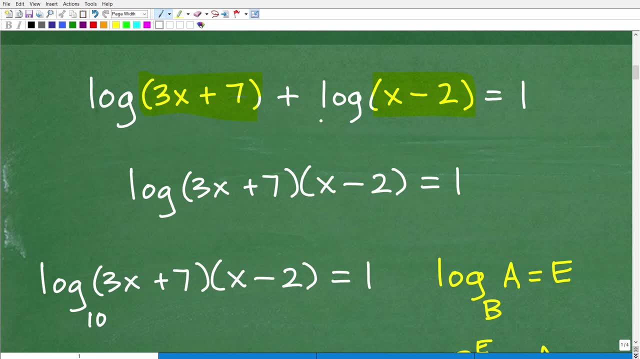 Now, one thing that you can have when you have LOG. okay, this is what we call the common log. the um here is actually base 10.. As long as these are the same, I can go ahead and condense this. 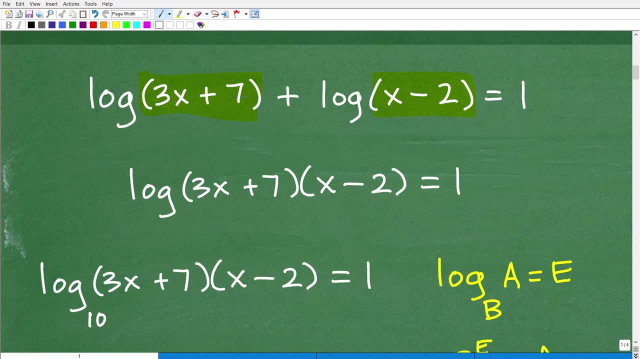 expression. In other words, I'm thinking: okay, this plus this- well, this must've came from log base 10 of three X plus seven times uh, um X minus two. Okay, So you can see that this is. 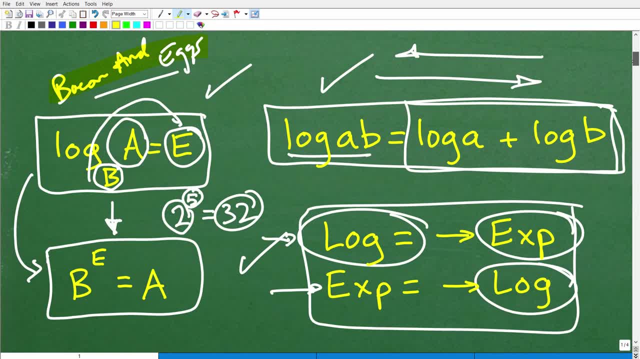 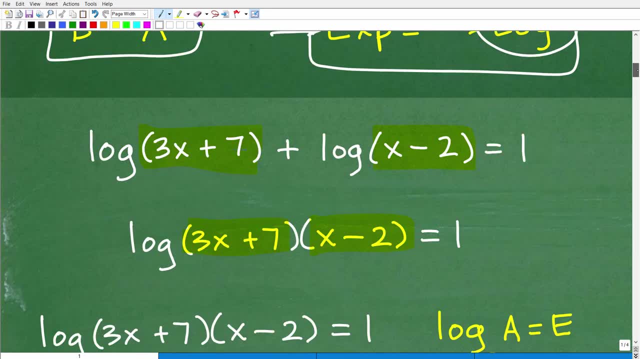 equivalent to this. Why? Because it's following this property of logarithms right here. Okay, We're just kind of condensing, We're going backwards. All right, You've got to be really good at condensing, Expanding, before you tackle these logarithmic equations, So hopefully you understand this is. 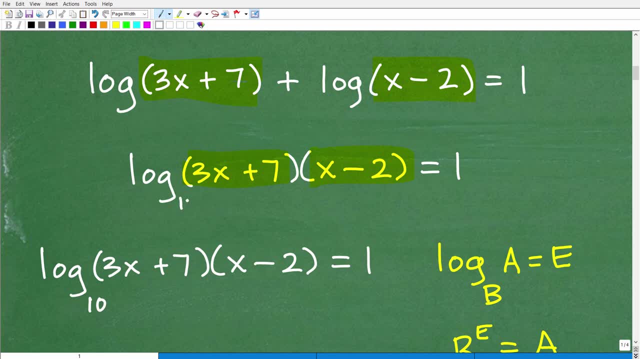 equal to this and that's equal to one. Okay, So now this is log base 10, just to be super clear about that- And the common logarithm. we don't typically write that base 10.. It's just implied that it's there. Okay, Now, uh, when you're dealing with a logarithmic equation, a logarithmic 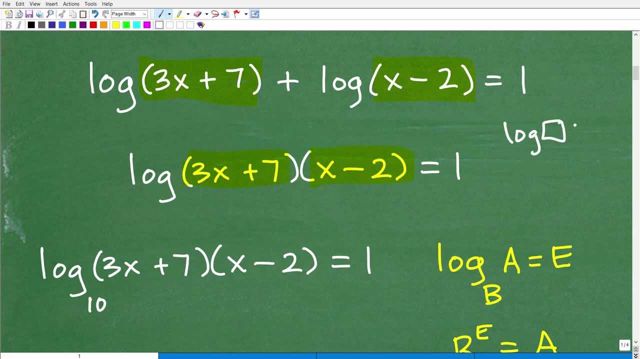 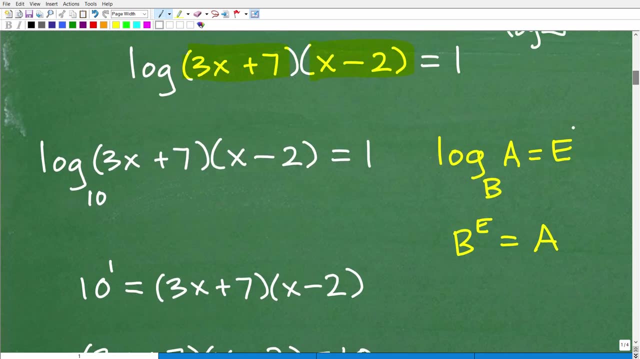 equation once you have your log uh part, all by itself equaling to like a number. now you're at a stage where you can rewrite this logarithmic uh expression or equation as a power. Okay, So the base- this is your bacon and eggs. Your base, that exponent is going to be equal to your answer. So 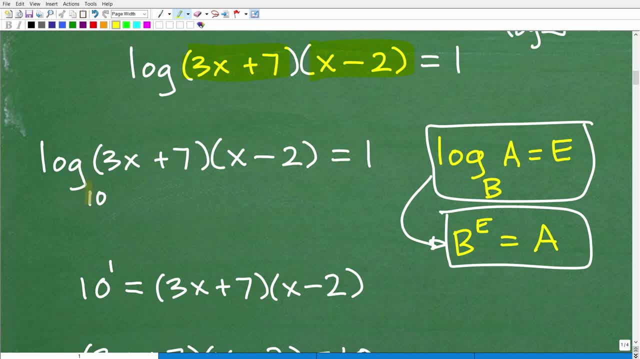 let's see how that is done now. So remember: log: the common log is base 10.. Okay, So this is the B. right here, This right here is the B. and then what is this? Okay, This part, this thing in front. 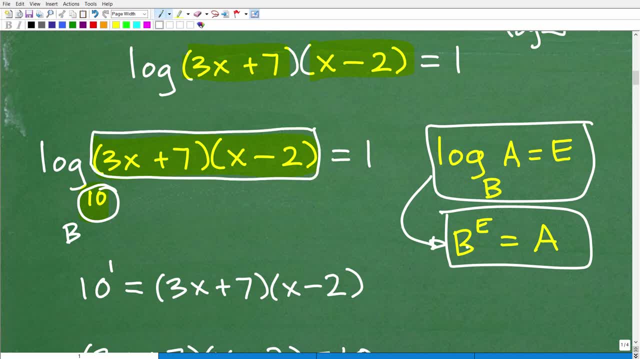 of the log. all of this stuff would be remember. this is the B, So that's the A. Okay, So this is the A and then that's going to be equal to the E, right here, That is the exponent. Okay, So the base to the exponent is equal to the answer. 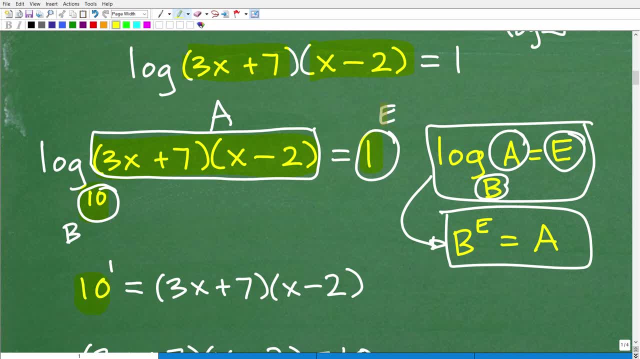 So let's go ahead and write that Now. the base is base 10. exponent is one: Okay, So 10 to the first Okay, I'm doing this right here- is equal to the answer, which is this: Okay, All right, So now. 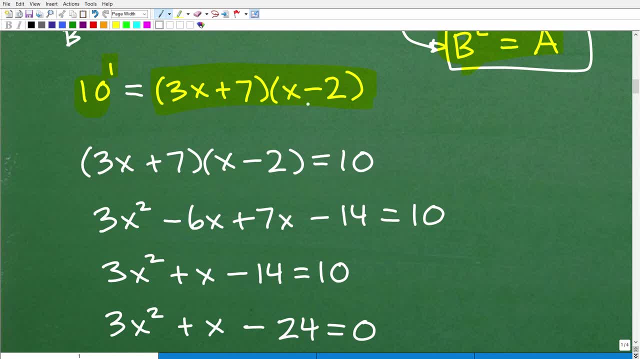 if I come to the şekа new and I go over here and I do a樣, and I do in the R prima for theriment mar Я на R sculptures, I'm going to do something like this. I'm going to do the R eliminate式. Okay. So now, 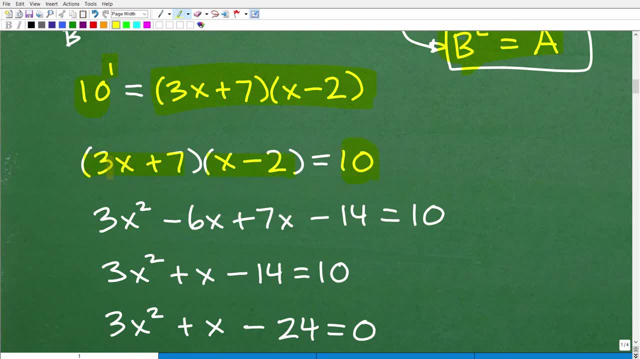 I got my first on. the first is equal to uh three X plus seven times uh X minus two. So it looks like I have a lovely quadratic equation. I mean this all. So this times this is equal to 10.. 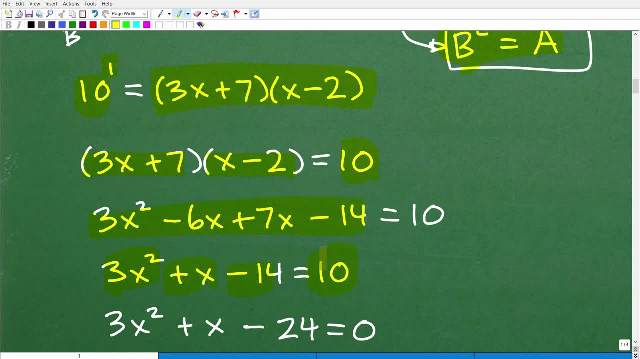 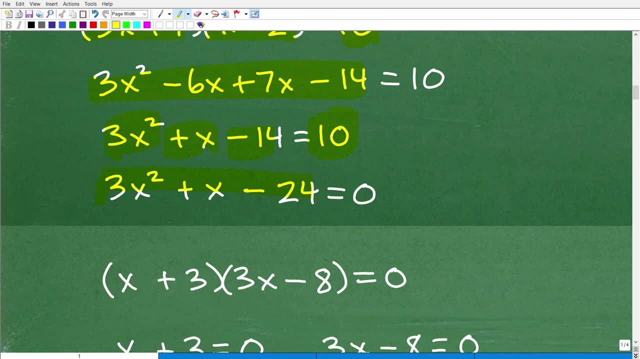 Well, when I need to do here is multiply, uh, these two mannan ewals. When I do that, I'm going to get three X squared plus X minus 14.. I'm just showing you. the work here is equal to 10.. So 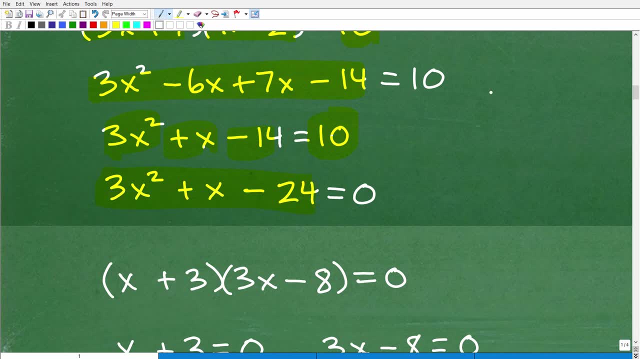 now I have to solve this quadratic equation, So I'm going to have to set this thing equal to zero. And you're like saying, Oh my goodness, I'm going to have to solve a quadratic equation. i thought it was just a logarithmic equation. yes, math builds upon itself and if you're at the level 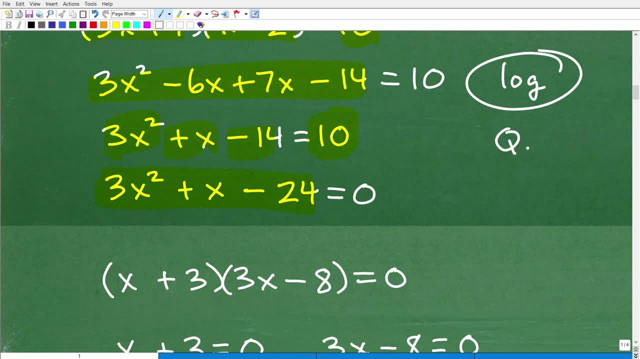 of solving logarithmic equations, you should have already mastered quadratic equations. so you're like: oh, i thought i uh, once i studied this, i don't have to remember it anymore. listen, i told you know, i don't know if you watched my other videos, but i'm telling you math is interconnected, so always. 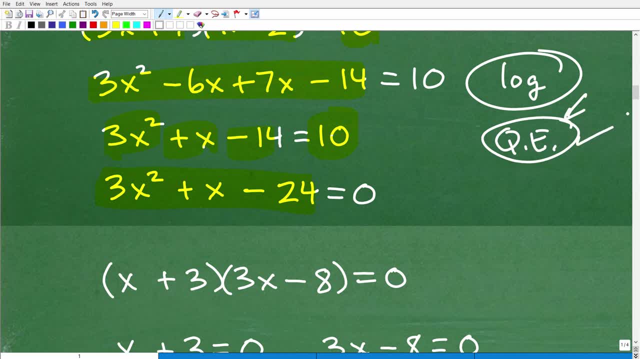 take well organized notes and you know there's really no shortcuts in math. so, yes, you're going to have to solve a quadratic equation here, so we're going to have to set this thing equal to zero. so i'm going to take this 10. move it over to the other side of the equation. subtract 10 from. 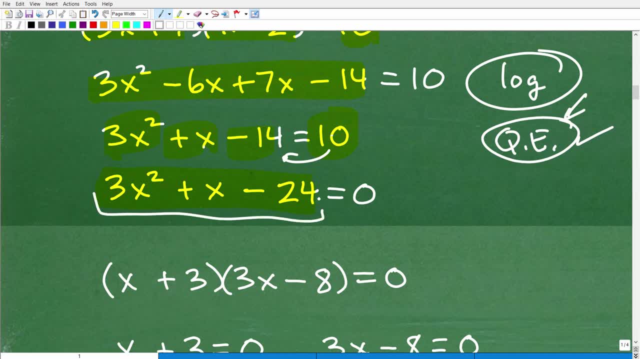 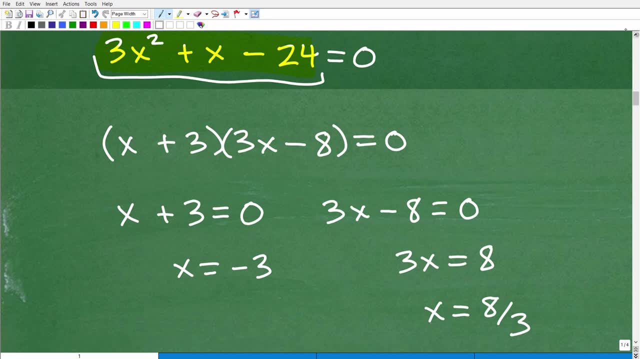 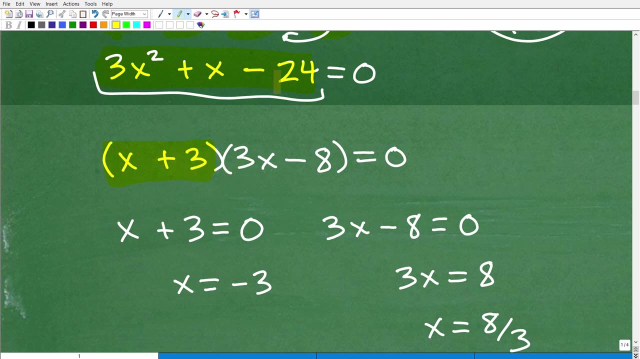 both sides equation. i get this: uh, trinomial 3x squared plus x minus 24 is equal to zero. okay, so what can i do here? well, luckily, this trinomial we can factor. we always want to try to factor. and uh, there's another skill that hopefully you know how to factor something. 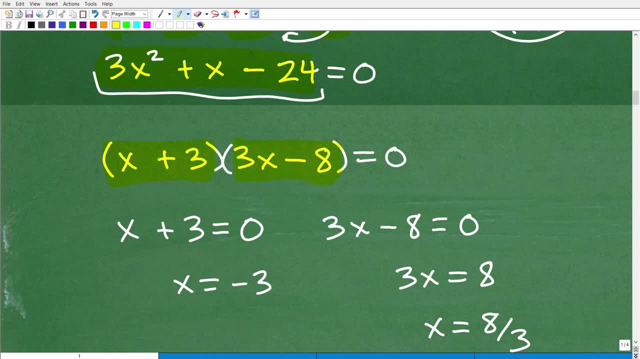 like this: that will be x plus 3 times uh, 3x minus 3x, squared plus x, squared squared plus x, squared squared squared squared squared minus 8. so solving quadratic equations involves the skill of factoring, very, very important. again, these are things that you will typically learn in algebra 1. what i'm doing right here is: 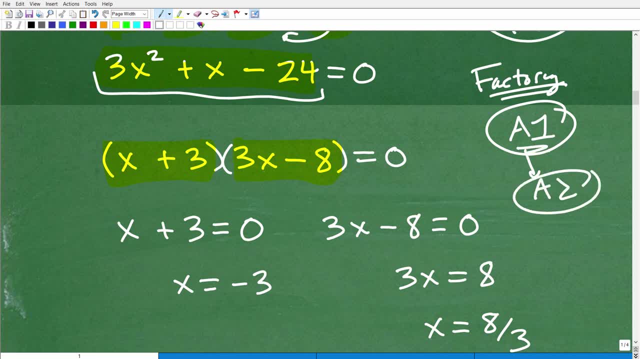 at like the algebra 2 level. so, um, you know, let's say you're at algebra 1 right now and you're just interested in this and you're- only, you know, doing, okay, well, algebra 2 is going to be much more difficult for you because you really have to master these skills. okay, and if you're in, 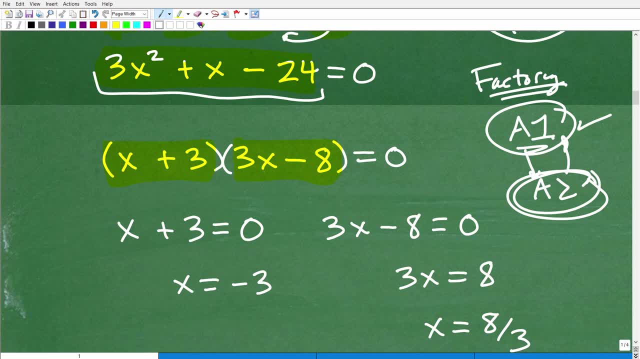 math. you can review and get really good at this stuff because you're going to need it. you know, uh, in algebra 2, college algebra, and definitely you know more advanced mathematics. okay, so we have x plus 3 times 3x minus 8 is equal to 0. now i can set each factor equal to 0, uh, so that's x plus 3. 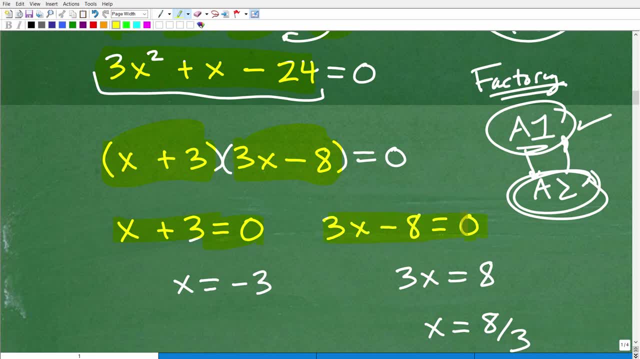 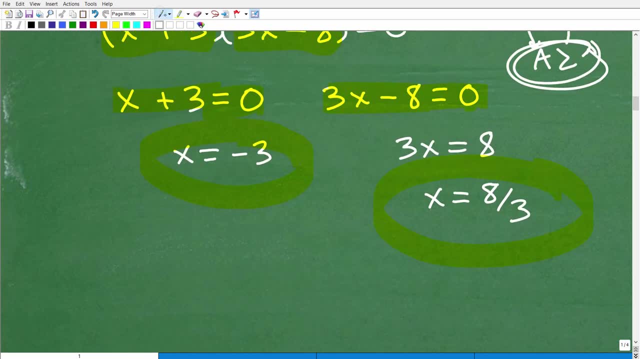 is equal to 0, and 3x minus 8 is equal to 0, and solve for x. so here i get: x is equal to negative 3. that's one solution. and here i get x is equal to 8 thirds. okay, so how did you do? did you actually? 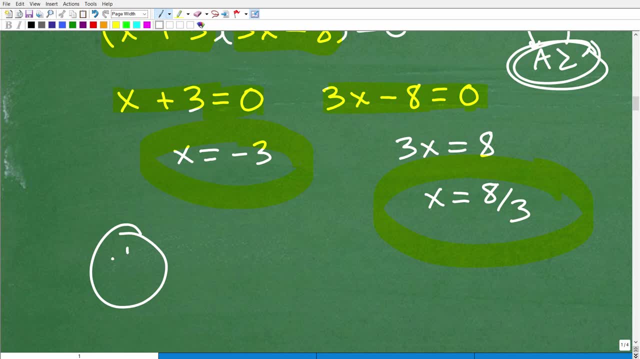 solve this problem all by yourself. well, if you did, i must give you a nice little happy face with a good old. 1986, that was a very good year. a flat top haircut and a plus a 120 percent and a few stars just to make you feel extra special today. that's pretty impressive, okay, uh, that's a. 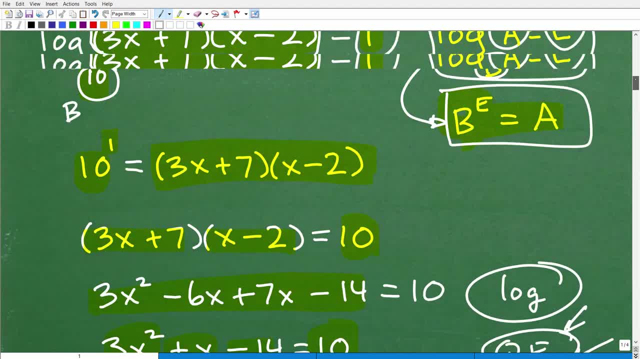 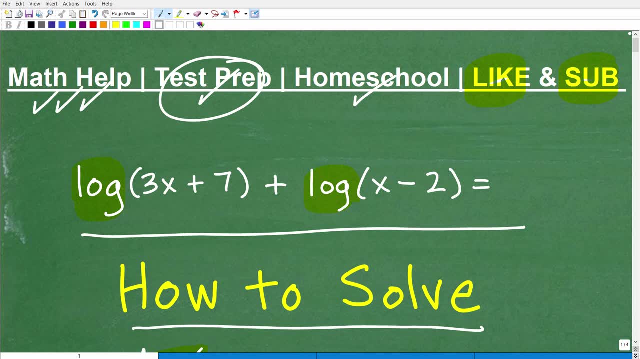 lot of you know knowledge contained here, but i would say this problem here, okay, is an average problem in terms of difficulty, okay. so if you're like, that's average, that was a lot of work. yeah, you're going to be doing much more challenging things than that, but, um, let's say you don't. 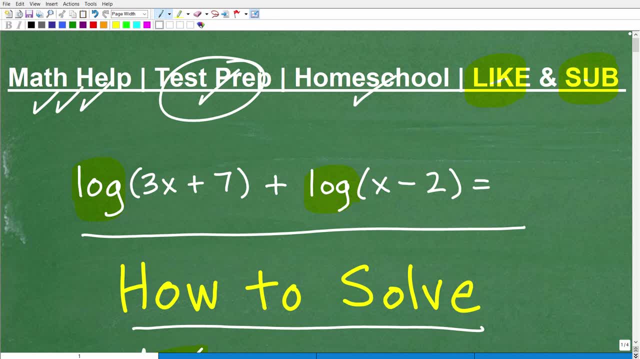 understand this. you're like overwhelmed. well, what do you do in terms of learning mathematics? well, if you're overwhelmed at this stage, you need to back up. you need to kind of look at the skills where you started, kind of getting lost, okay, and typically what ends up happening is that a lot of 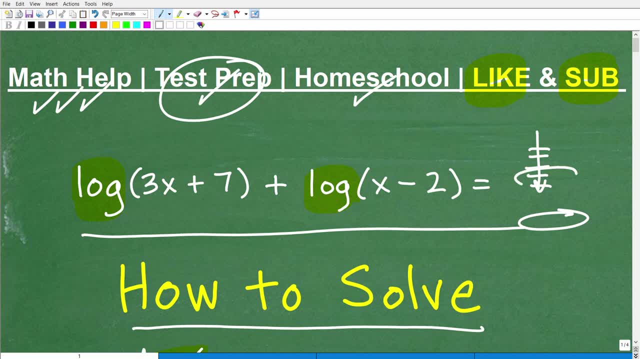 students struggle with things. in the past they forgot how to factor they're. they don't really know how to solve quadratic equations. they don't understand the big picture about logarithmic equations, exponential functions, etc. so that's why it's so important to get your you know um great math instruction. you know. hopefully you got a great teacher, but if you 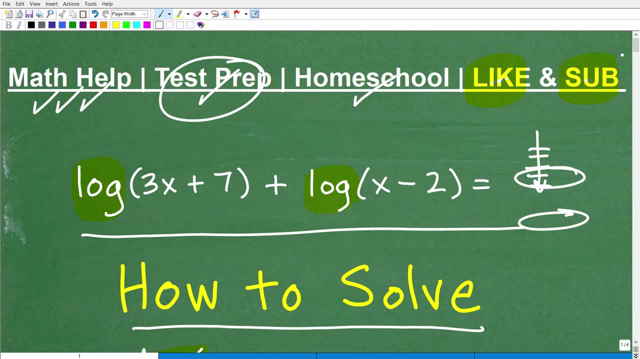 you know if you're not really connecting with your teacher, you know, use a program like mine or someone else's so you can really comprehend and master these concepts, because at this level of math it's going to get much more involved and all these topics are interrelated, but the bottom line is you. 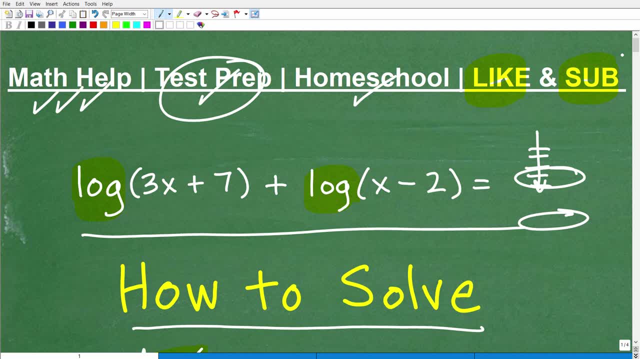 are going to have to work harder than others, but everyone can be successful in mathematics and hopefully this video helped you out again. if that was the case, but smash that like button and subscribe to my youtube channel, all right. so, with that being said, i definitely wish you all the best. in your mathematics adventures. thank you for your time and have a great day.